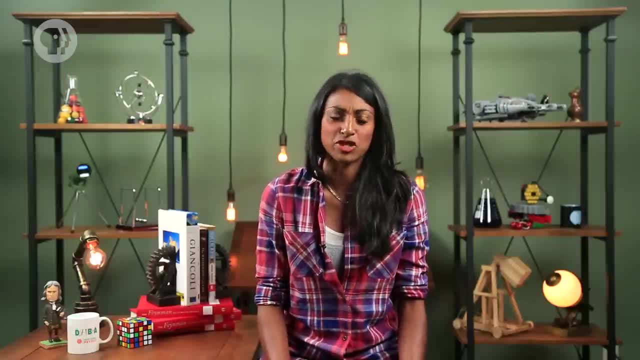 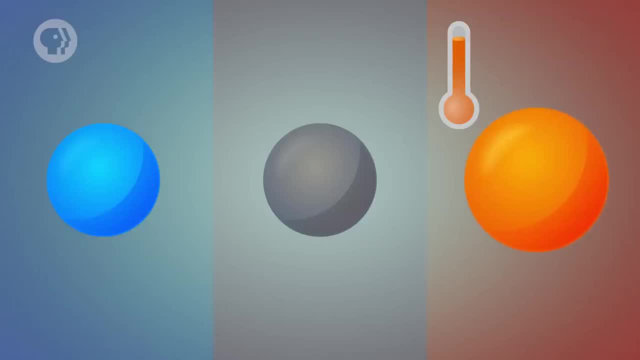 But usually there will be some heat transfer, because that's how the temperature of a system works, And when the temperature of an object changes, it can undergo what's known as thermal expansion. Usually, an increase in temperature will make a solid expand and a decrease in temperature will make it contract. 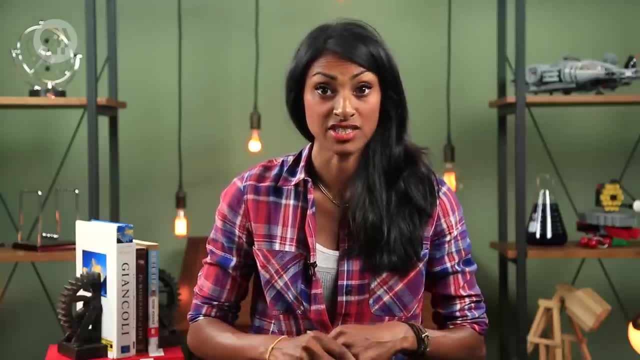 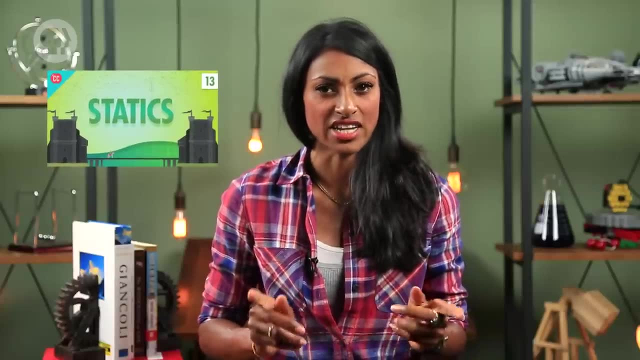 Now there are two main ways that the dimensions of a solid can change based on a change in temperature. It can increase or decrease in length, or it can increase or decrease in volume. These changes in length and volume work in a very similar way to the changes in length and volume from stress and strain. 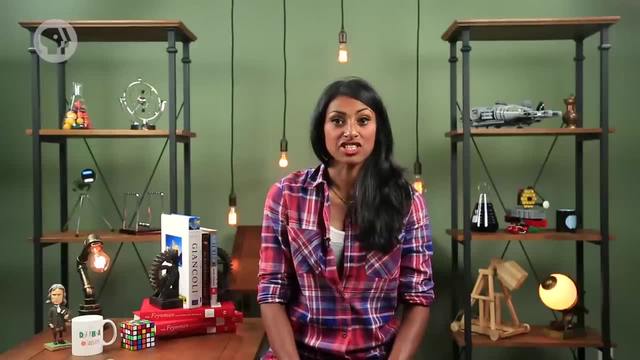 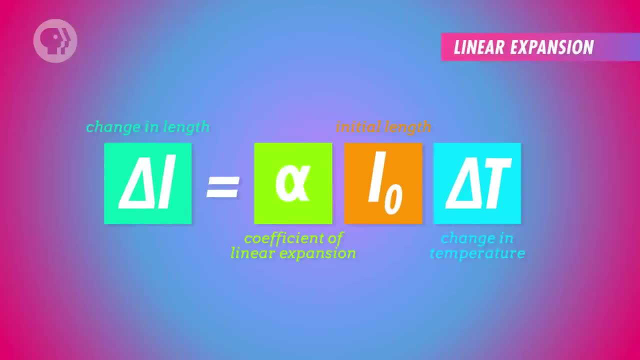 that we talked about in our episode on statics. In the case of a bridge, the change is in its length, what's known as linear expansion- And the equation that we used to describe linear expansion says that the change in length is equal to what's known as the coefficient of linear expansion. 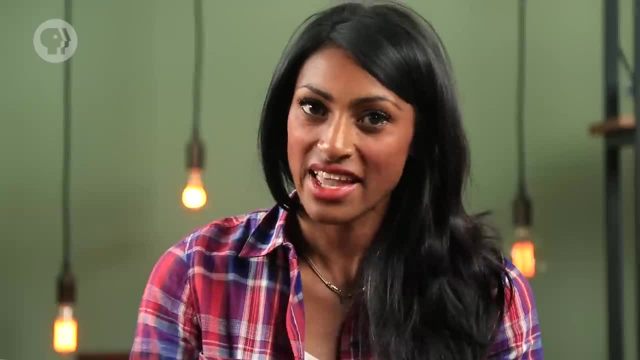 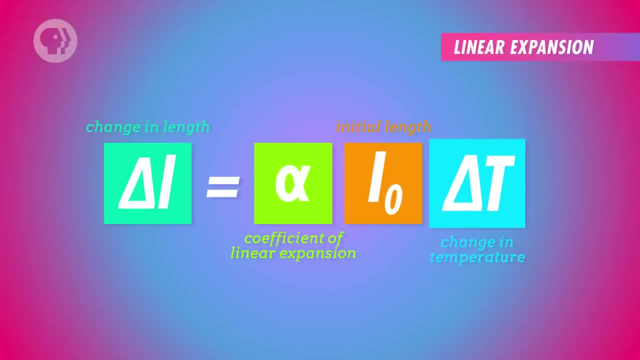 times the initial length, times the change in temperature. So let's break that equation down to see how it works. The longer the bridge is to start with, the more it will expand or contract, and the greater the temperature change, the more it will also expand or contract. 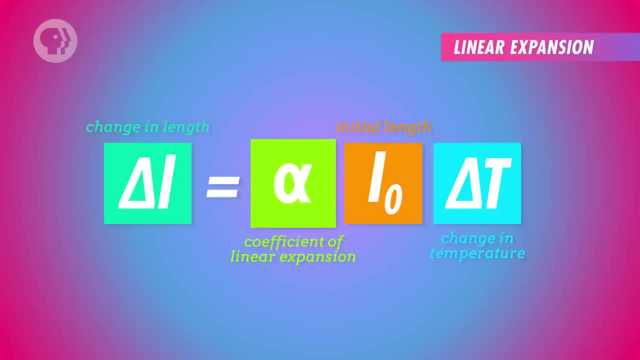 The only other thing that the change in length depends on is that coefficient of linear expansion, represented by the Greek letter alpha. The value for that coefficient depends on the material, and the higher the coefficient, the more it will expand or contract, The more the length of the material will change in response to a change in temperature. 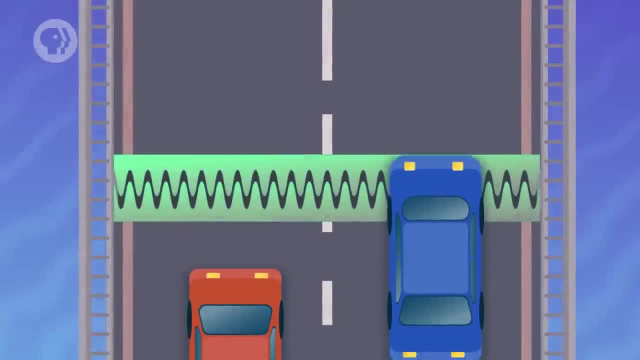 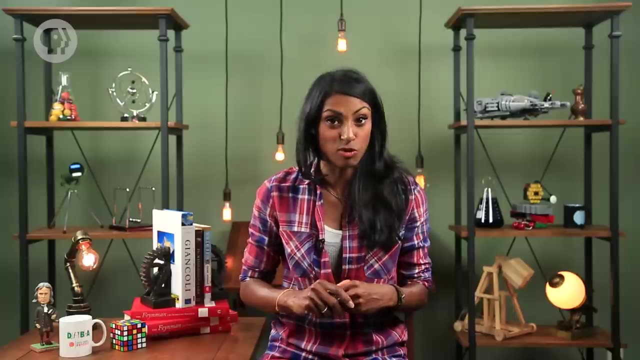 And that's why bridges have expansion joints: to give the concrete room to expand when it's warmer outside and contract back down in cooler weather. Without expansion joints, the concrete would experience much more stress and you'd be much more likely to end up with a broken bridge. 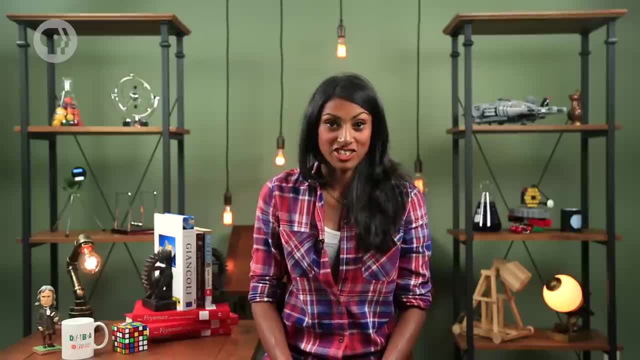 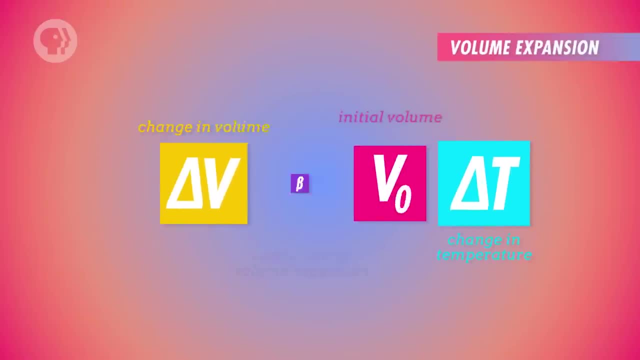 And the same principles apply to other kinds of expansion. Volume expansion is just like linear expansion, except that the change happens in all three dimensions. The equation for volume expansion just says that the change in volume is equal to the coefficient of volume expansion times the initial volume, times the change in temperature. 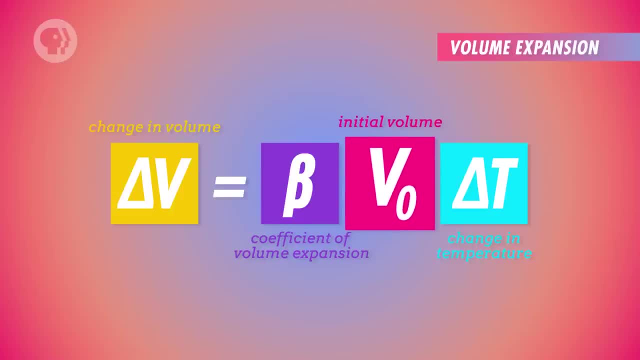 As with linear expansion, the bigger the object is in the first place, the more it will expand or contract, And a greater temperature change will lead to a greater change in volume. Finally, the volume change depends on how much of a tendency any particular material has to expand or contract. 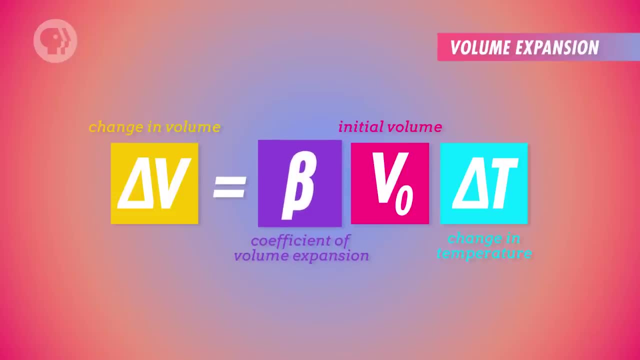 That is coefficient of volume expansion, represented by the Greek letter beta. But changes in temperature don't only affect solids, they also affect gases And in gases temperature has to be equal to the coefficient of volume expansion times the initial volume times the change in temperature. 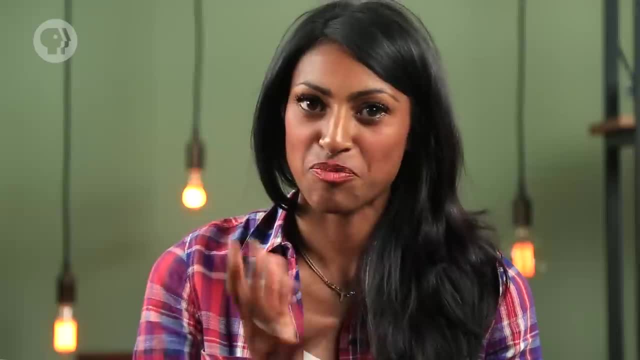 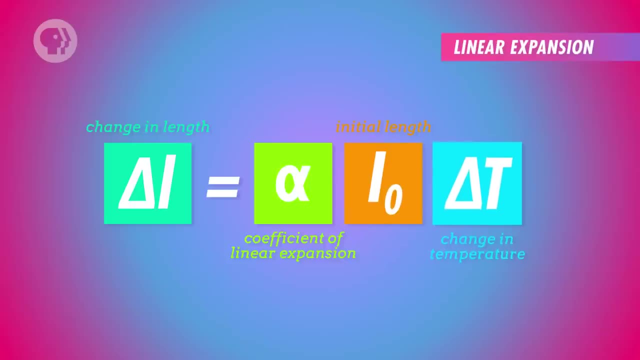 times the initial length, times the change in temperature. So let's break that equation down to see how it works. The longer the bridge is to start with, the more it will expand or contract, and the greater the temperature change, the more it will also expand or contract. 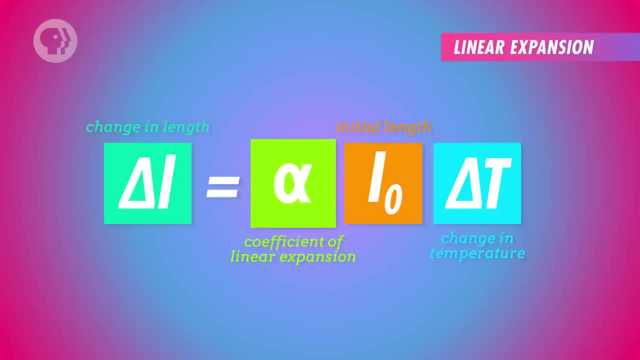 The only other thing that the change in length depends on is that coefficient of linear expansion, represented by the Greek letter alpha. The value for that coefficient depends on the material, and the higher the coefficient, the higher the value, The more efficient it is, the more the length of the material will change in response to a change in temperature. 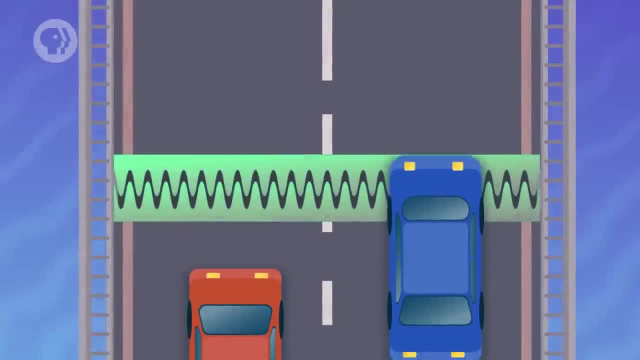 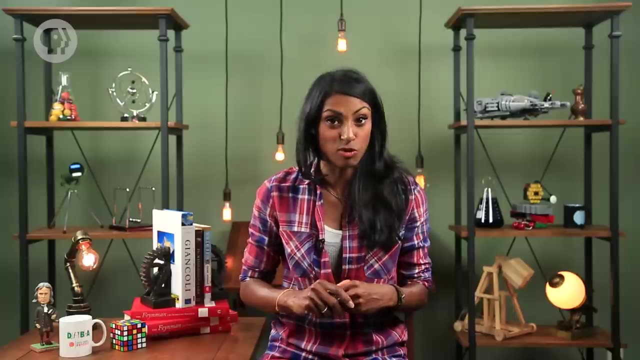 And that's why bridges have expansion joints: to give the concrete room to expand when it's warmer outside and contract back down in cooler weather. Without expansion joints, the concrete would experience much more stress and you'd be much more likely to end up with a broken bridge. 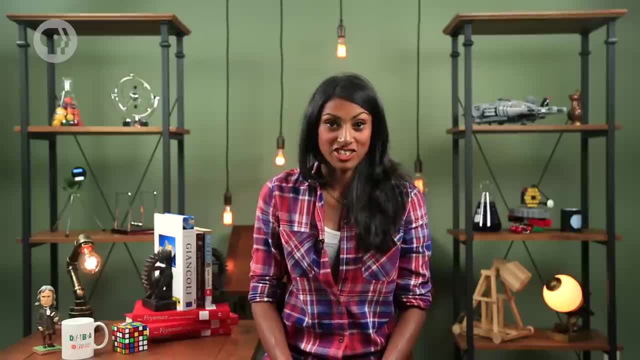 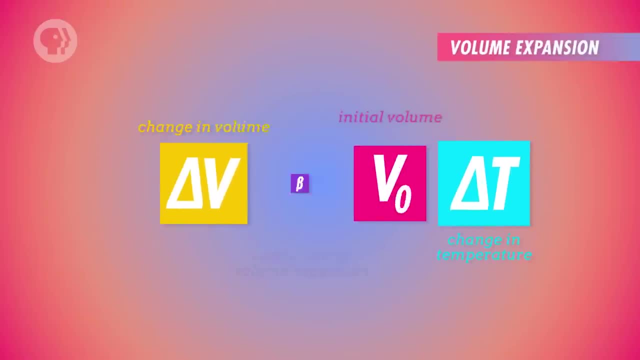 And the same principles apply to other kinds of expansion. Volume expansion is just like linear expansion, except that the change happens in all three dimensions. The equation for volume expansion just says that the change in volume is equal to the coefficient of volume expansion times the initial volume, times the change in temperature. 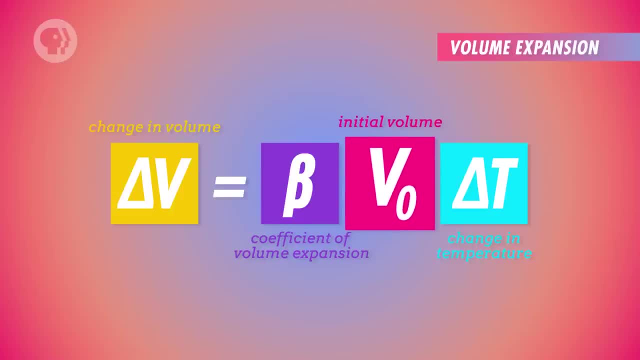 As with linear expansion, the bigger the object is in the first place, the more it'll expand or contract, And a greater temperature change will lead to a greater change in volume. Finally, the volume change depends on how much of a tendency any particular material has to expand or contract. 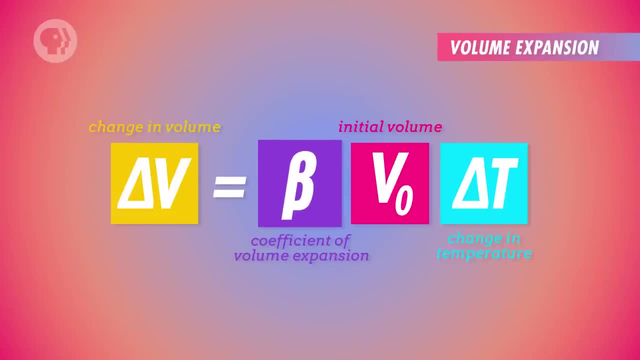 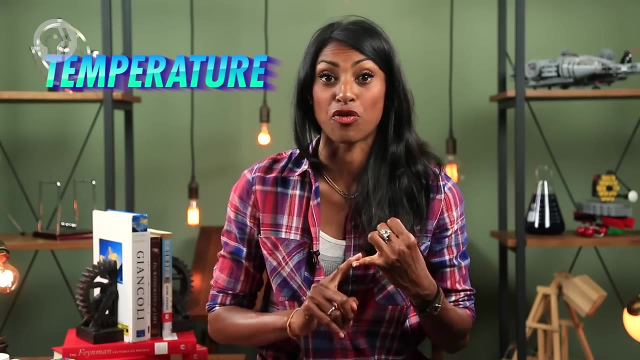 That is coefficient of volume expansion, represented by the Greek letter beta. But changes in temperature don't only affect solids, they also affect gases And in gases temperature has to be equal to the coefficient of volume. expansion has a direct bearing on the pressure, volume and amount of the gas. 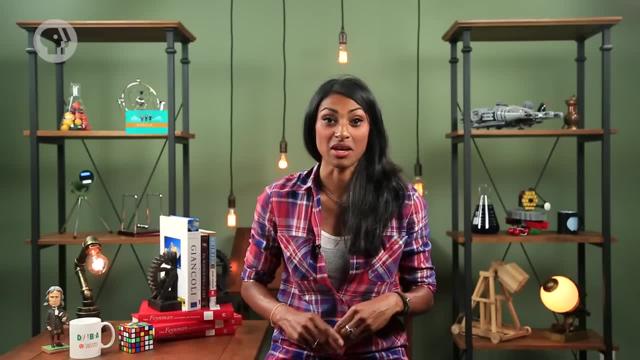 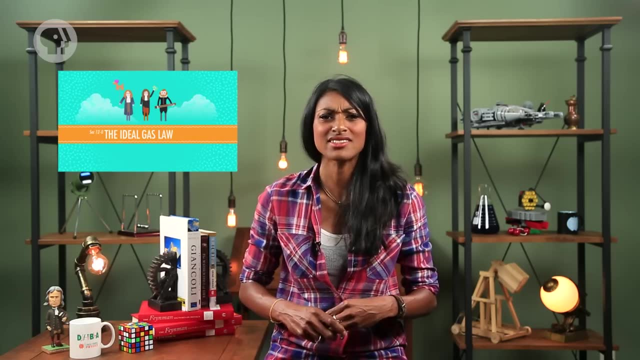 All four of these properties are related to one another. If you've taken a chemistry course, like maybe the one Hank hosted, you're probably already familiar with the concept of an ideal gas, a hypothetical gas that obeys a certain set of rules, which lets you describe it more simply. So what are these rules? Well, an ideal gas is made up of lots of molecules that move around randomly. As they're zooming around, those molecules might collide and bounce off one another, but they'll exert no other forces on each other outside of these collisions. 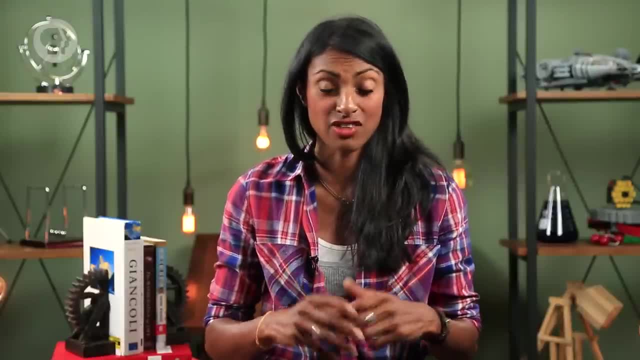 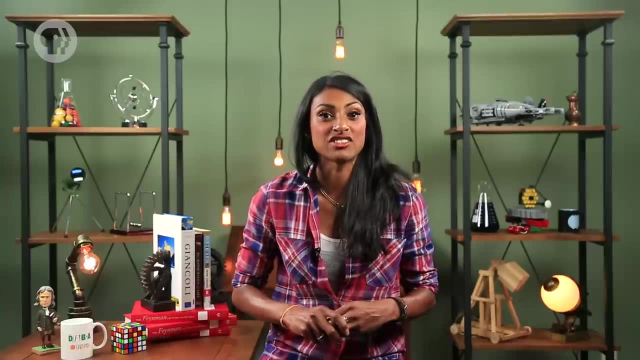 And the volume of all the gas molecules combined is very small compared to the volume of the container, And in many cases, a real gas is close enough to an ideal gas that these assumptions apply, Which means that we can use the equations that describe ideal gases to describe the 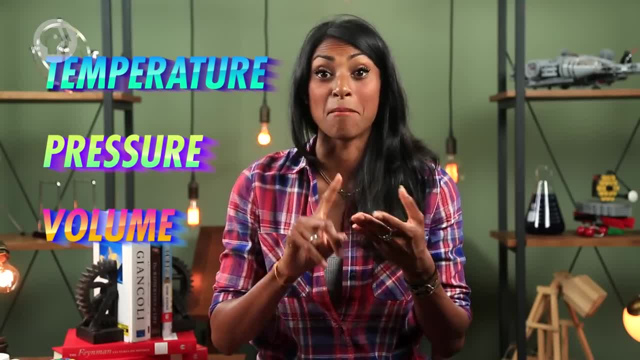 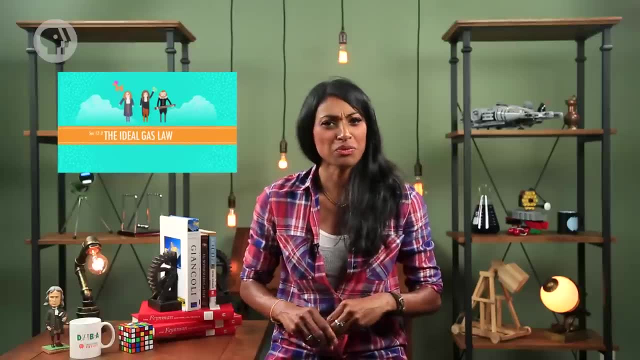 In other words, temperature has a direct bearing on the pressure, volume and amount of the gas. All four of these properties are related to one another. If you've taken a chemistry course, like maybe the one Hank hosted, you're probably already familiar with the concept of an ideal gas. 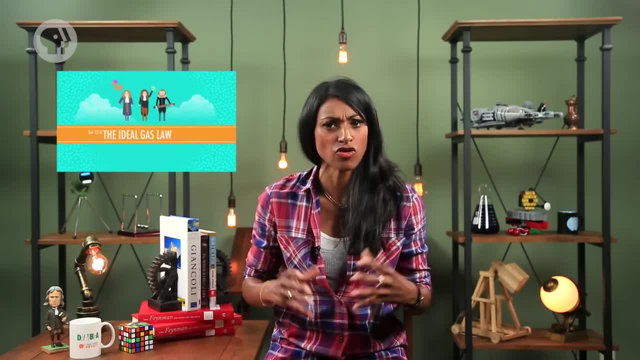 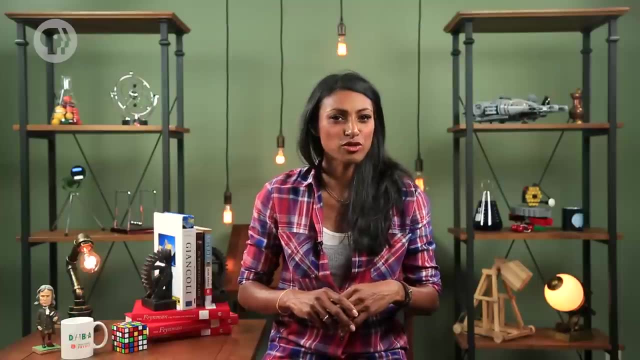 A hypothetical gas that obeys a certain set of rules, which lets you describe it more simply. So what are these rules? Well, an ideal gas is made up of lots of molecules that move around randomly. As they're zooming around, those molecules might collide and bounce off one another, but they'll exert no other forces on each other outside of these collisions. 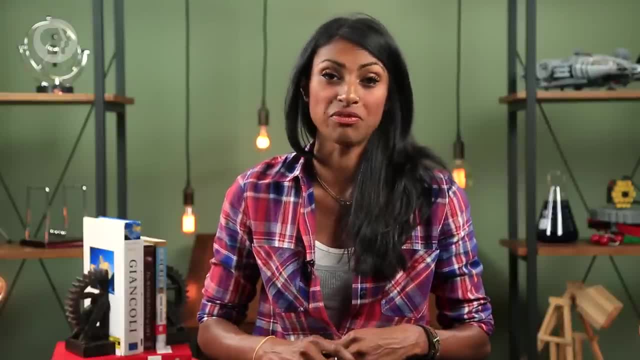 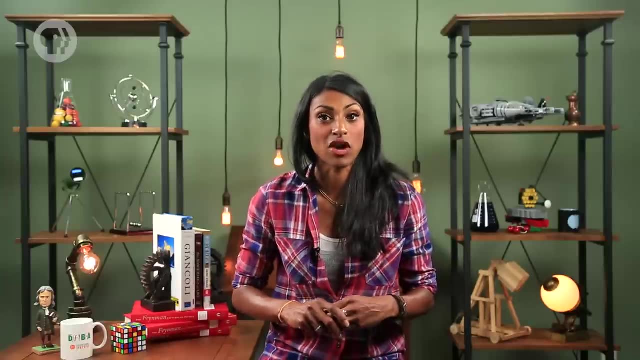 The volume of all the gas molecules combined is very small compared to the volume of the container, And in many cases a real gas is close enough to an ideal gas that these assumptions apply, Which means that we can use the equations that describe ideal gases to describe the behavior of lots of real-life situations too. 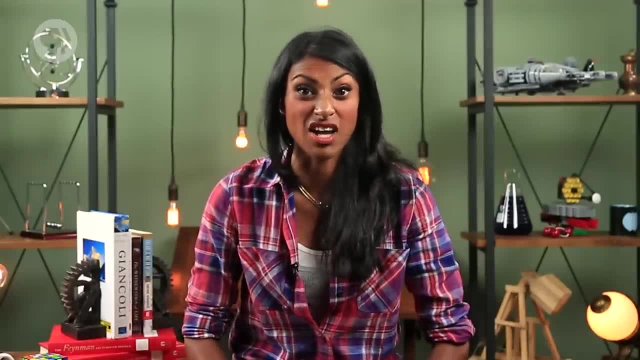 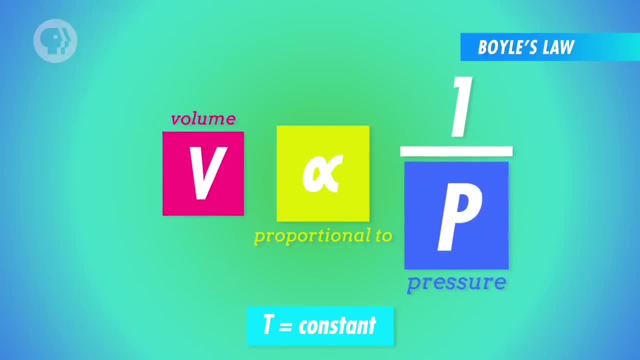 And each of these laws is named after a uniquely awesome individual who lived hundreds of years ago. The first is called Boyle's Law and it says that as you increase the pressure of a gas while holding the temperature constant, the volume of the gas will go down, and vice versa. 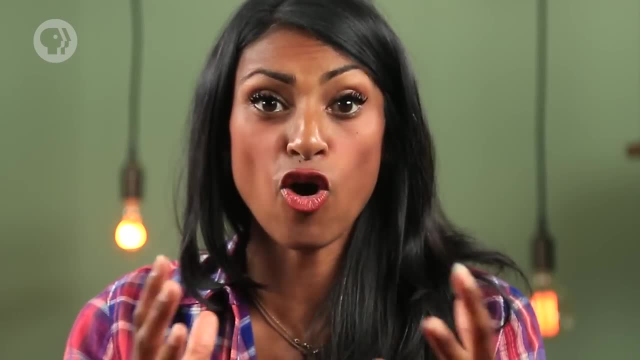 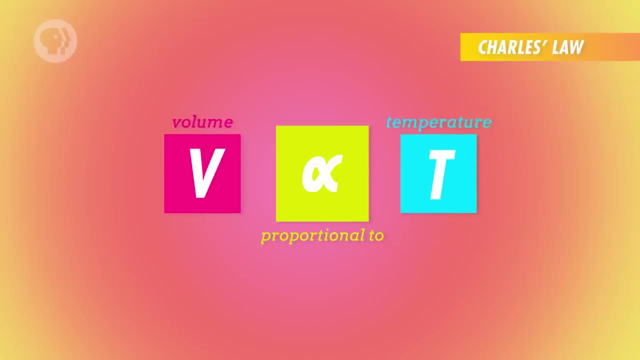 When you increase the pressure, you're squeezing the molecules together so they occupy less space. The second basic law is called Charles' Law, and it says that as you increase the temperature of a gas while holding the pressure constant, the volume of the gas will go up, and vice versa. 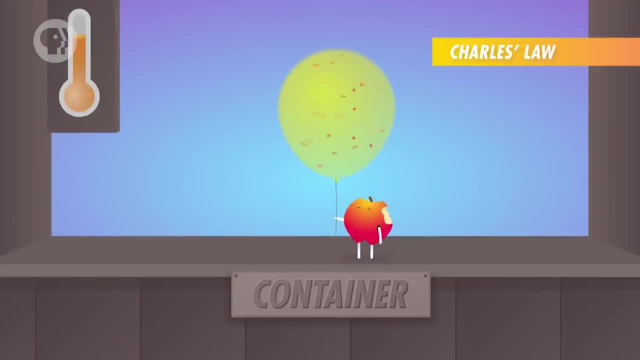 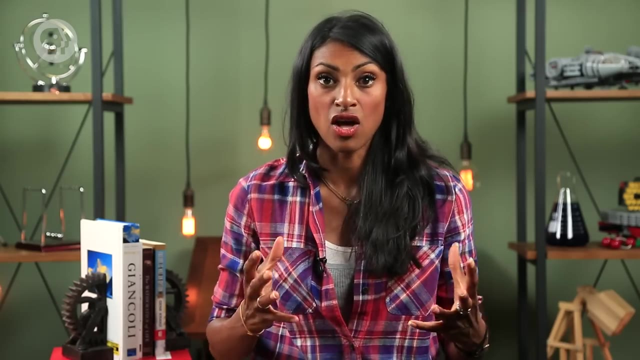 Raising the temperature of the gas gives the molecules more energy, which means they can rocket around more forcefully, expanding the size of the container. So far, we've talked about how the properties of an ideal gas relate to each other when you hold the temperature constant and when you hold the pressure constant. 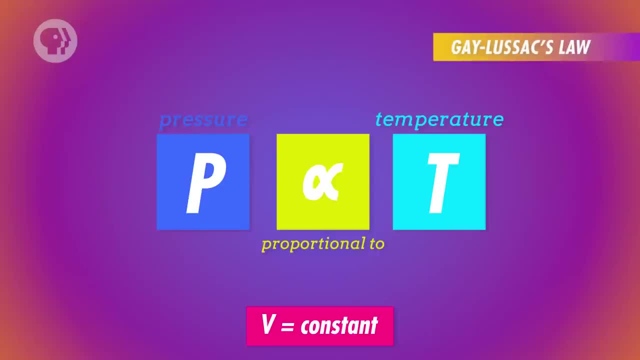 So you can probably guess what the third law is for. It's called Gay-Lussac's Law, and it says that if you increase the temperature of a gas while holding the volume constant, the pressure of the gas will go up, and vice versa. What's happening here is that the increase in temperature again gives the gas molecules more energy and a higher speed, but this time the size of the container is fixed, So the molecules hit the side of the container more often and with more force, increasing the pressure inside. 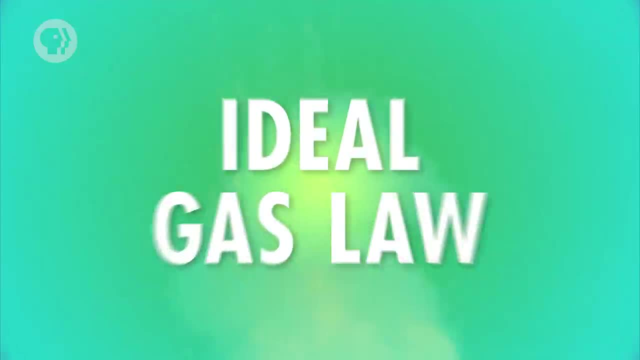 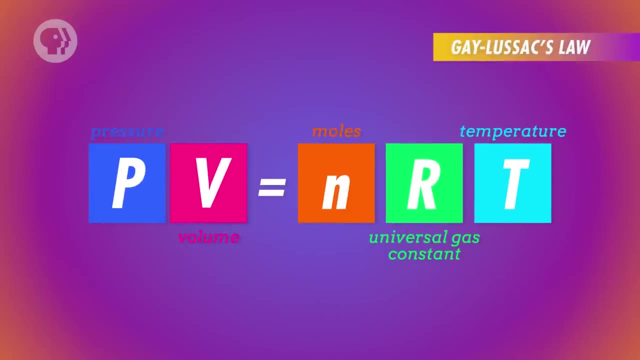 All three of these laws can be combined into one main equation, known simply as the ideal gas law, which also takes into account the amount of the gas Pressure times. volume is equal to the number of moles in the gas times. R times. the temperature, also known as PV, equals nRT. 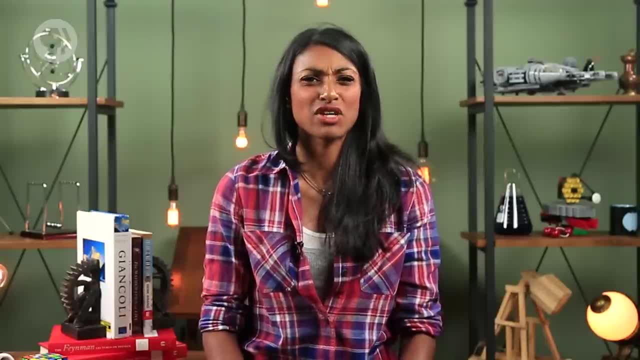 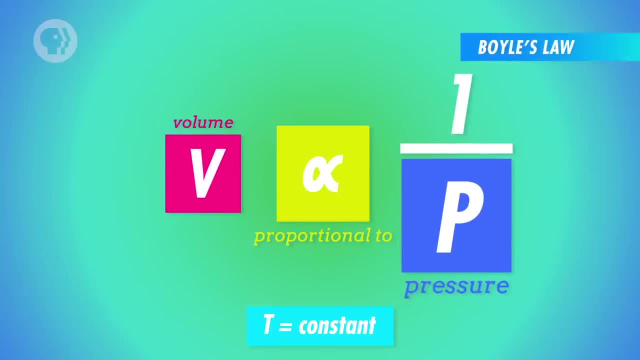 behavior, of lots of real-life situations too, And each of these laws is named after a uniquely awesome individual who lived hundreds of years ago. The first is called Boyle's Law, and it says that as you increase the pressure of a gas while holding the temperature constant, the volume of the gas will go down, and vice versa. 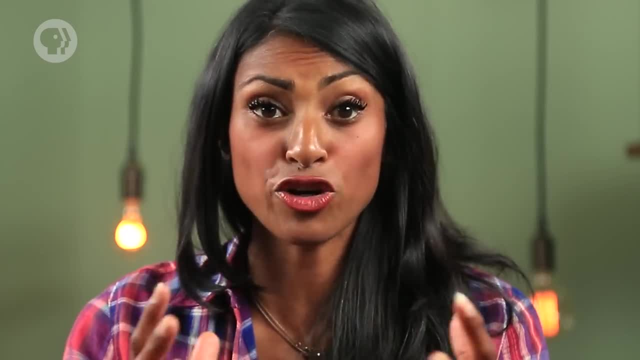 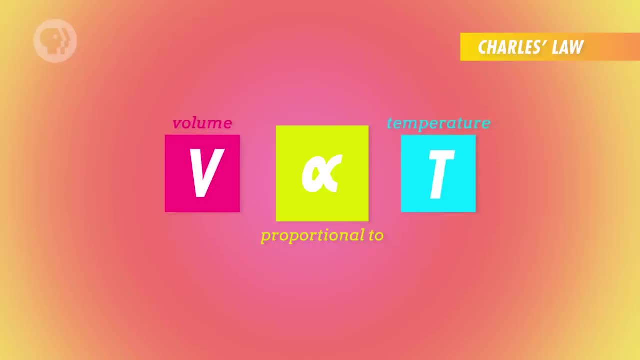 When you increase the pressure, you're squeezing the molecules together so they occupy less space. The second basic law is called Charles' Law, and it says that as you increase the temperature of a gas while holding the pressure constant, the volume of the gas will go up, and vice versa. 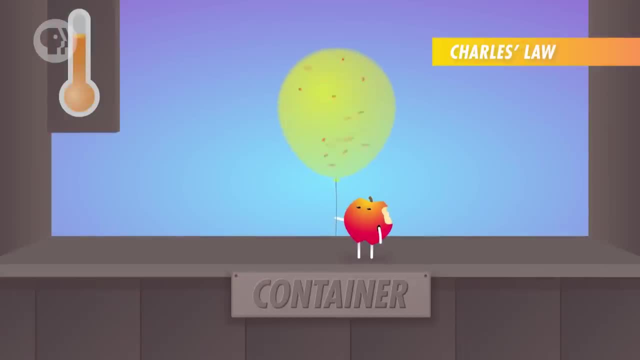 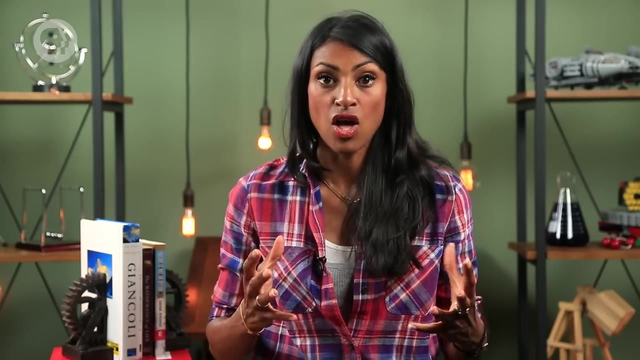 Raising the temperature of the gas gives the molecules more energy, which means they can rocket around more forcefully, expanding the size of the container. So far, we've talked about how the properties of an ideal gas relate to each other when you hold the temperature constant and when you hold the pressure constant. 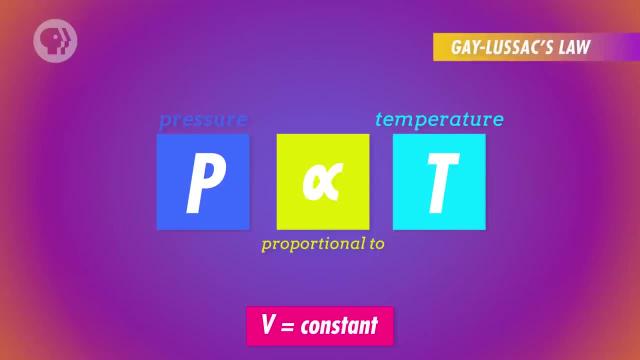 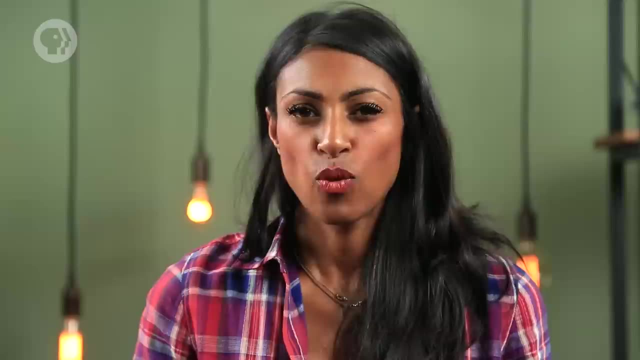 So you can probably guess what the third law is for. It's called Gay-Lussacian Law, And it says that if you increase the temperature of a gas while holding the volume constant, the pressure of the gas will go up, and vice versa. What's happening here is that the increase in temperature again gives the gas molecules more energy and a higher speed, but this time the size of the container is fixed, So the molecules hit the side of the container more often and with more force increasing. 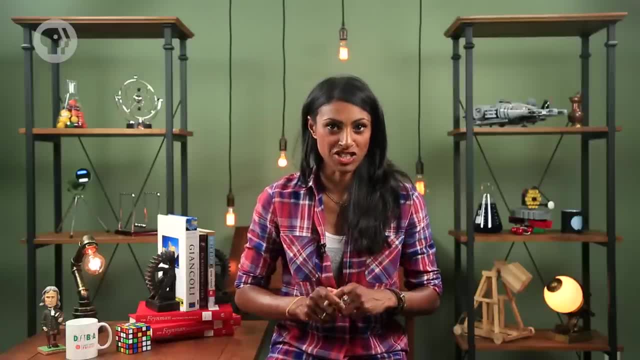 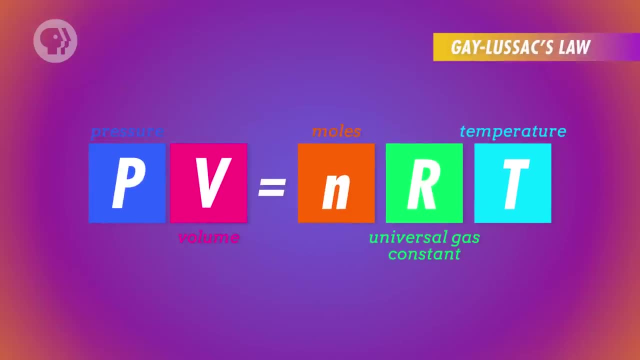 the pressure inside. All three of these laws can be combined into one main equation, known simply as the ideal gas law, which also takes into account the amount of the gas Pressure times. volume is equal to the volume of the gas Pressure times. volume is equal to the number of moles in the gas times. R times the temperature. 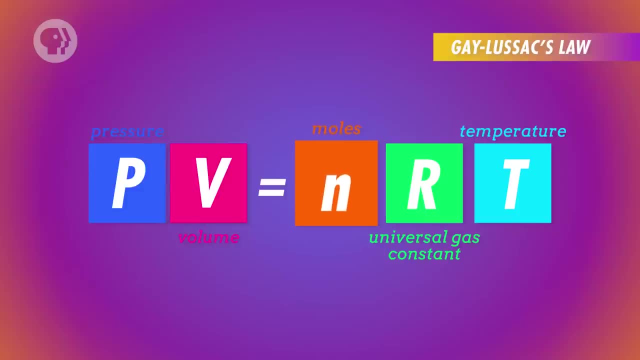 Also known as PV, equals nRT. The N stands for the number of moles of the gas. A mole is just a unit that's used to measure the amount of a substance, in this case a gas, in terms of the number of molecules. 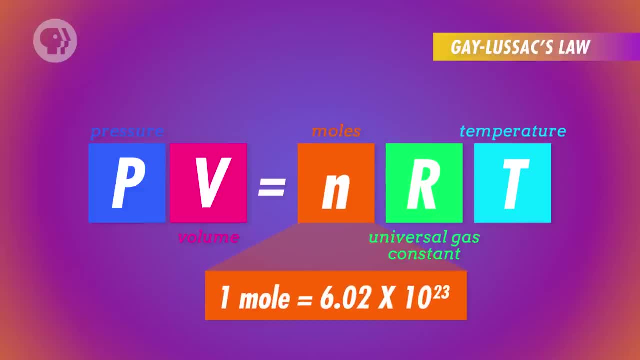 If you have one mole of gas, it means that you have 6.02 times 10 to the 23 molecules of the stuff. R, meanwhile, is what's called the universal gas constant. It's a number that connects the pressure and volume of an ideal gas to the number of. 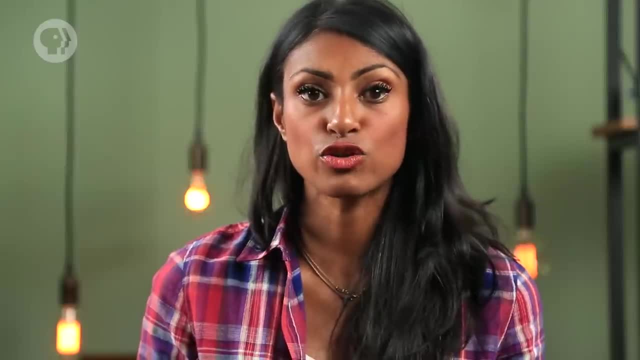 moles of the gas and its temperature. And for every ideal gas, as long as your unit is equal to the number of moles of the gas you have, 6.02 times 10 to the 23 molecules of the stuff. If your units are consistent, R will be exactly the same number. 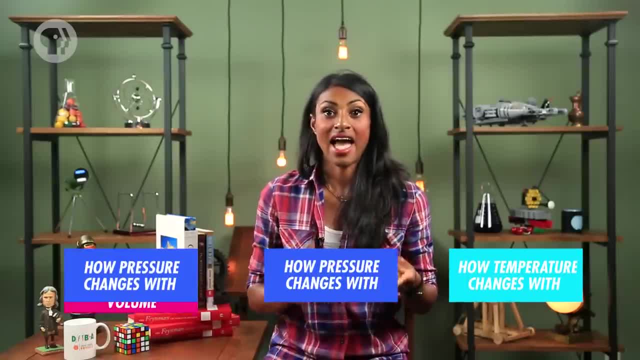 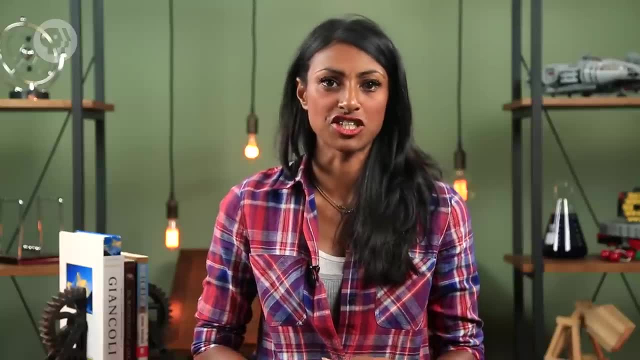 The ideal gas law includes the three basic laws we just talked about: How pressure changes with volume, how temperature changes with volume and how pressure changes with temperature. But instead of talking about each of those relationships individually, it lets you relate all four properties of a gas, including how much gas you have. 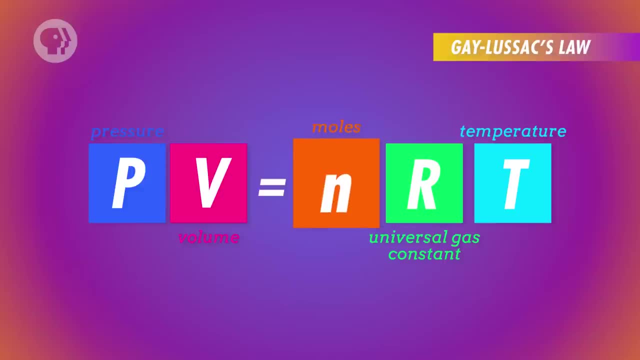 The N stands for the number of moles of the gas. A mole is just a unit that's used to measure the amount of a substance, in this case a gas. in terms of the number of molecules, If you have one mole of gas, it means that you have 6.02 times 10 to the 23 molecules of the stuff. 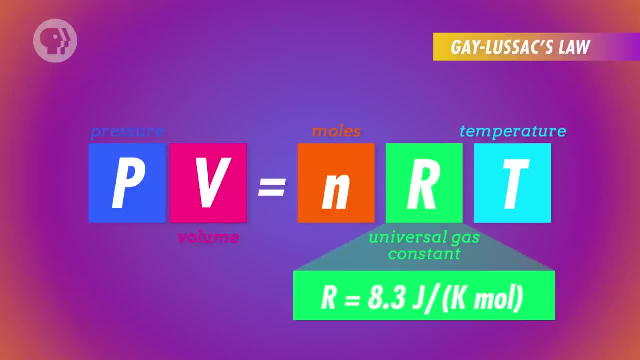 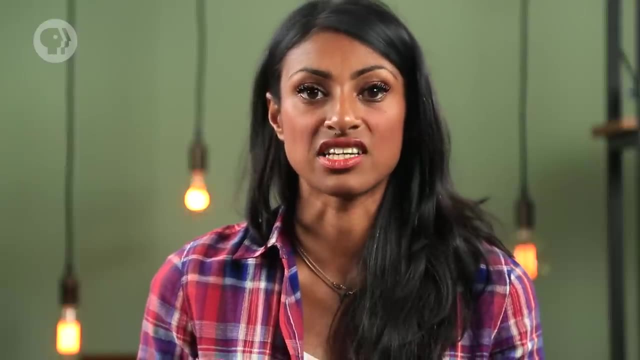 R, meanwhile, is what's called the universal gas constant. It's a number that connects the pressure and volume of an ideal gas to the number of moles of the gas and its temperature, And for every ideal gas, as long as your units are consistent, R will be exactly the same number. 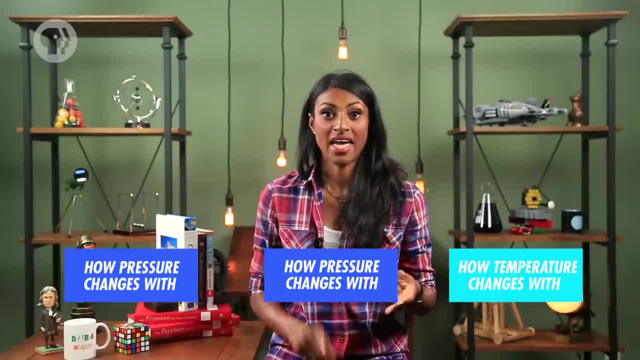 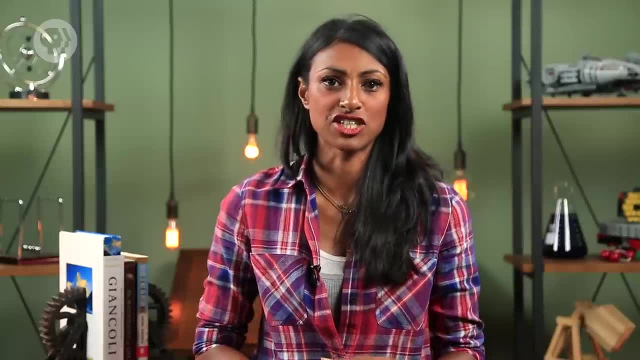 The ideal gas law includes the three basic laws we just talked about – how pressure changes with volume, how temperature changes with volume and how pressure changes with temperature. But instead of talking about each of those relationships individually, it lets you relate all four properties of a gas, including how much gas you have. 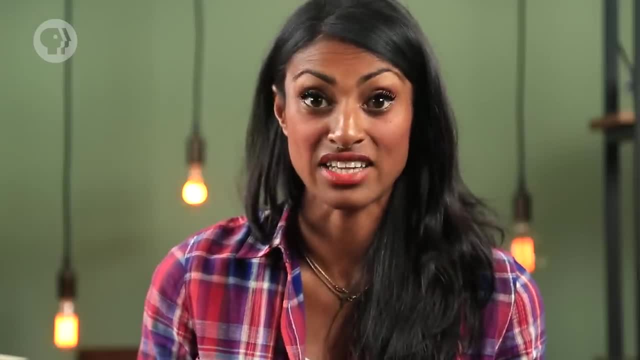 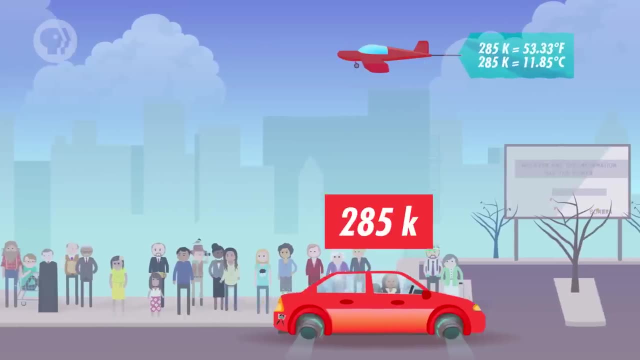 To see all of this in action, let's consider how the ideal gas law relates to your commute. Let's say that, as part of your daily routine, you drive to school once in the morning and once in the afternoon. It's pretty chilly in your car as you drive in the morning – about 285 Kelvin – and you don't bother to turn on the heat. 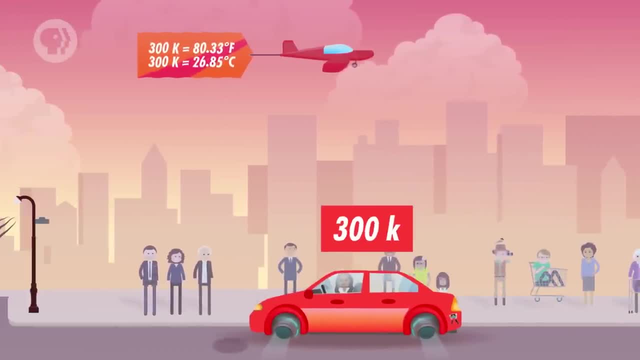 By the time the afternoon comes along, it's much warmer in your car – about 300 Kelvin – but you don't turn on the air conditioning. What we want to know is how many fewer moles of air there are in your car in the afternoon. 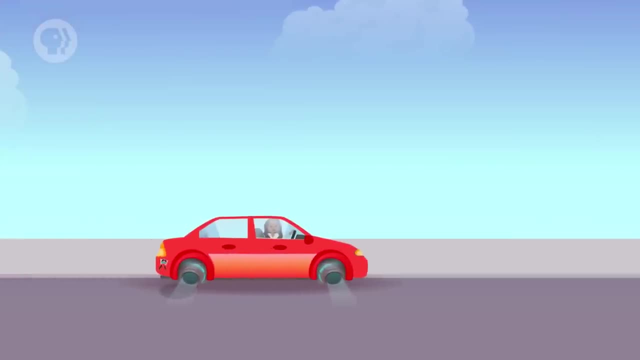 Your car isn't airtight, so molecules of air are free to move in and out. Laws say that the volume of the inside of your car where you sit is about 5 meters cubed, and that volume isn't going to change much. 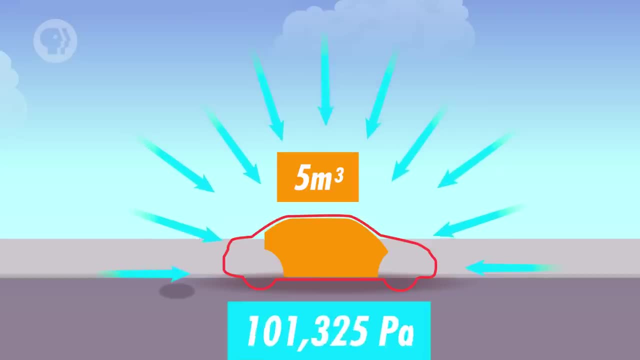 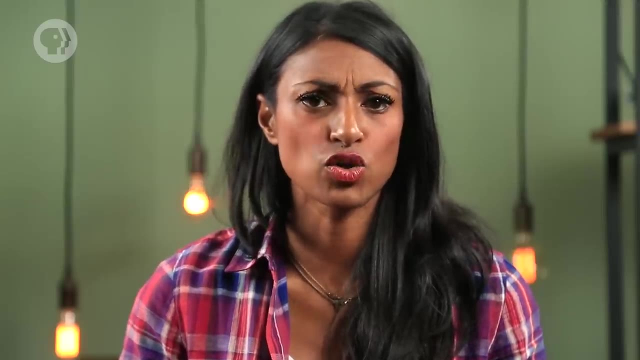 The pressure inside your car is going to be equal to the outside air pressure, Which we'll take to be the standard atmospheric pressure, or 101,325 Pascals. So how many moles of air were inside your car as you drove to class in the morning? 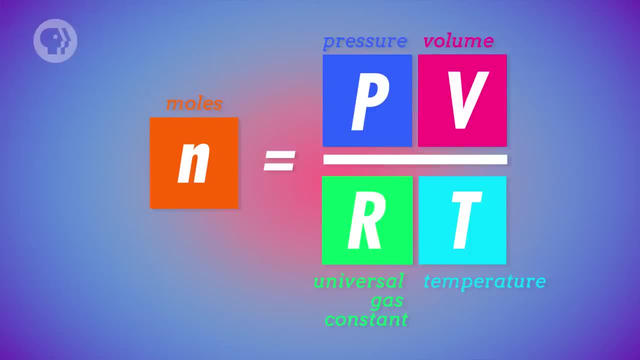 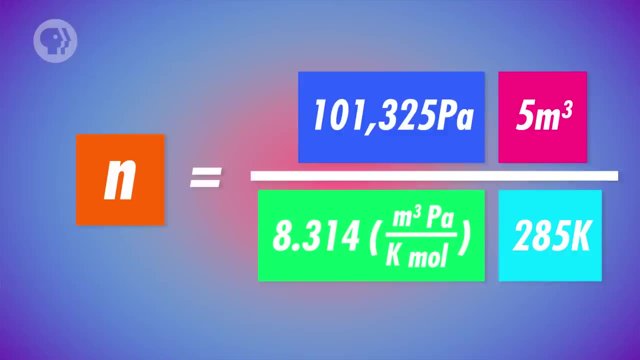 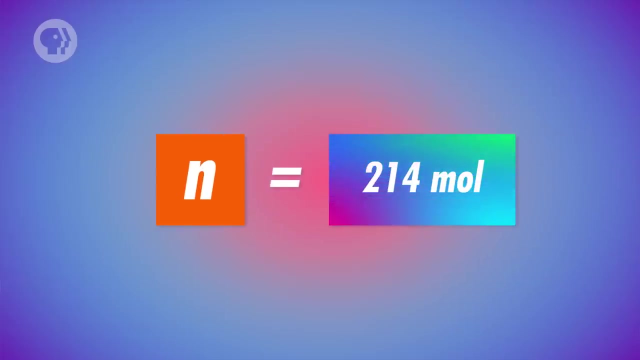 Well, according to the ideal gas law, the amount of gas in moles is equal to pressure times volume divided by temperature times, the universal gas constant, And 101,325 Pascals times 5 meters cubed divided by the universal gas constant times, 285 Kelvin is about 214 moles. 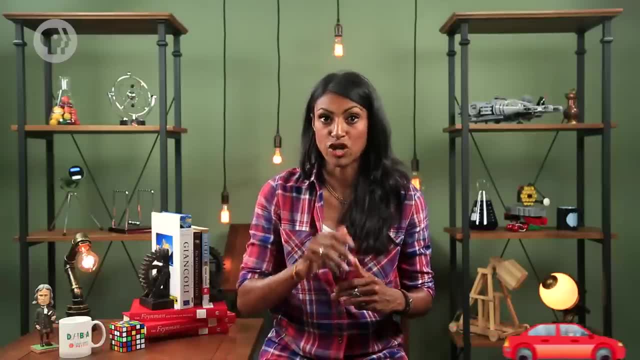 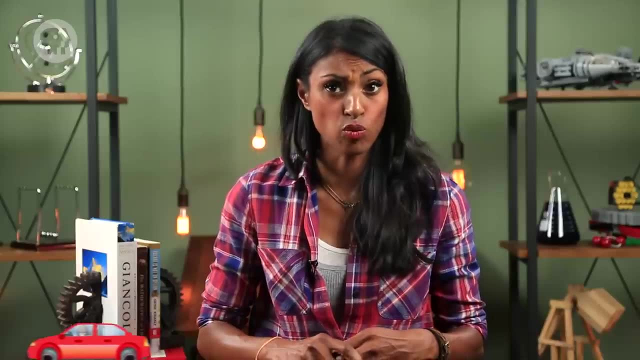 So there are roughly 214 moles. So how many moles of air were inside your car when you drove to class in the morning? Now, how many moles of air were inside your car when you drove home in the afternoon, when it was about 15 Kelvin warmer than in the morning? 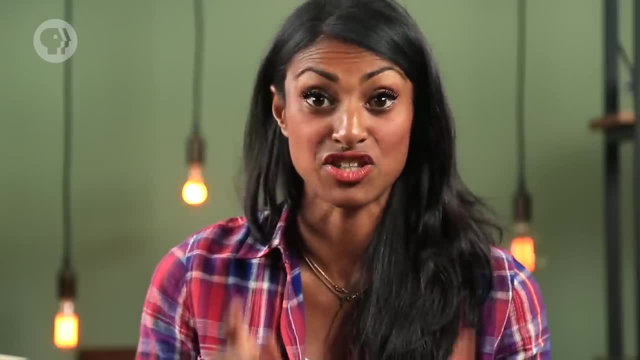 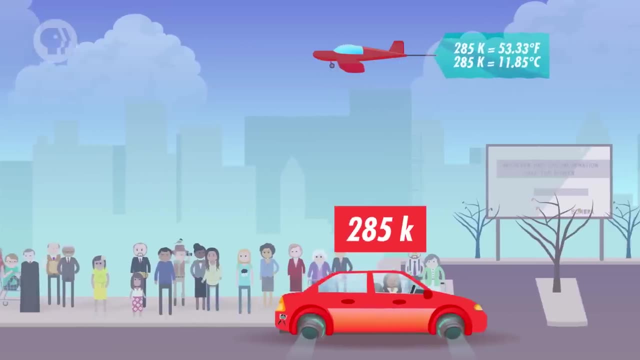 To see all of this in action, let's consider how the ideal gas law relates to your commute. Let's say that as part of your daily routine, you drive to school once in the morning and once in the afternoon. It's pretty chilly in your car as you drive in the morning- about 285 Kelvin and you. 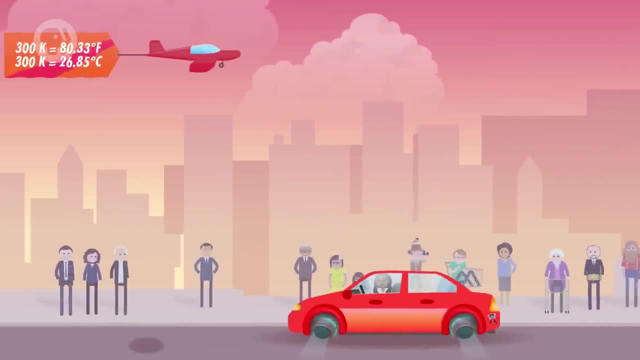 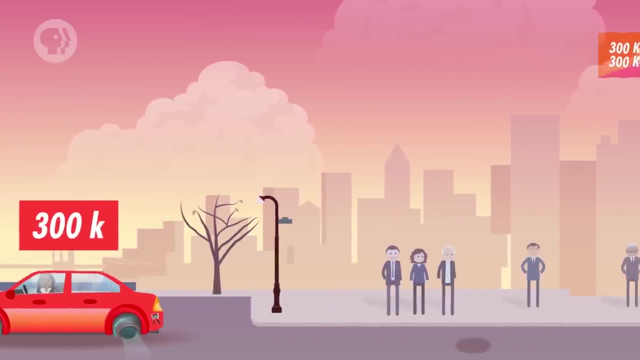 don't bother to turn on the heat. By the time the afternoon comes along, it's much warmer in your car- about 300 Kelvin- but you don't turn on the air conditioning. What we want to know is how many fewer moles of air there are in your car in the afternoon. 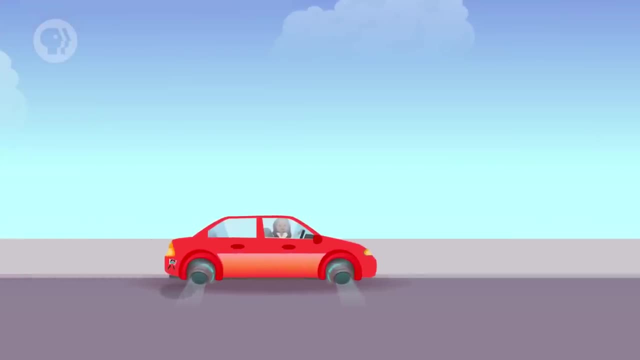 Your car isn't airtight, so molecules of air are free to move in and out. Laws say that the volume of the inside of your car where you sit is about 5 meters cubed, and that volume isn't going to change much. 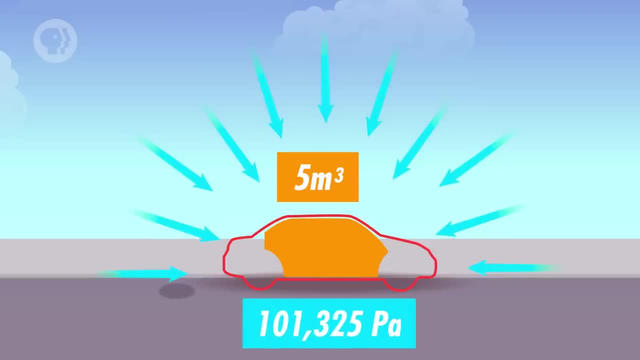 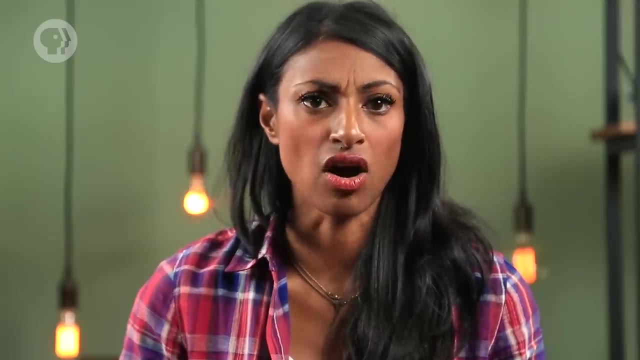 The pressure inside your car is going to be equal to the outside air pressure, which will take to be the standard atmospheric pressure, or 101,325 Pascals. So how many moles of air were inside your car as you drove to class in the morning? 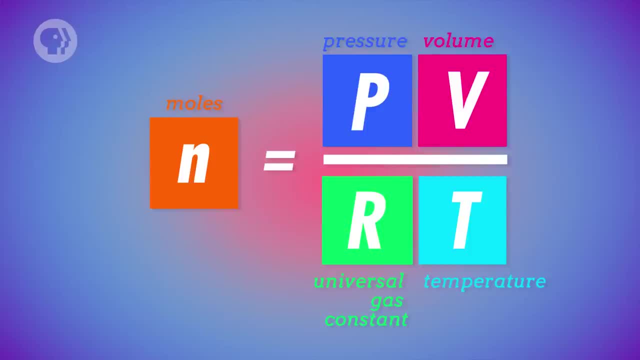 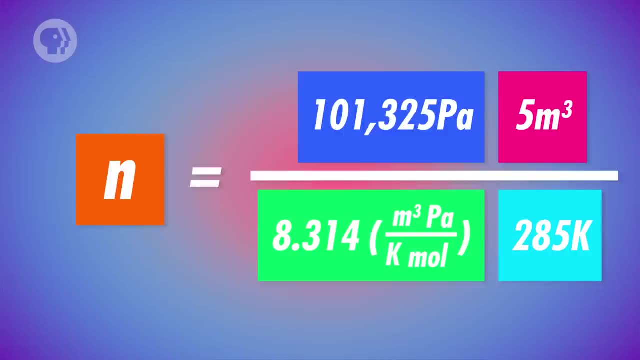 Well, according to the ideal gas law, the amount of gas in moles is equal to pressure times volume divided by temperature times the universal gas constant And 101,325 Pascals times 5 meters cubed divided by the universal gas constant times 285 Kelvin. 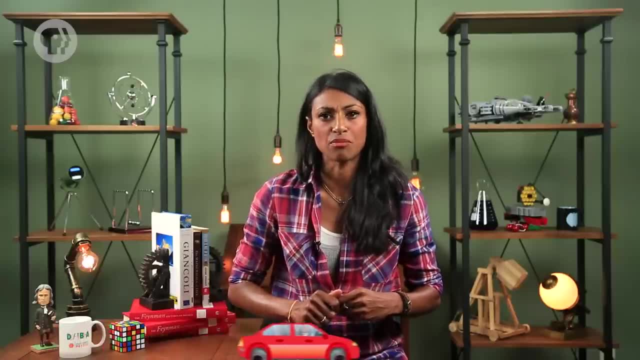 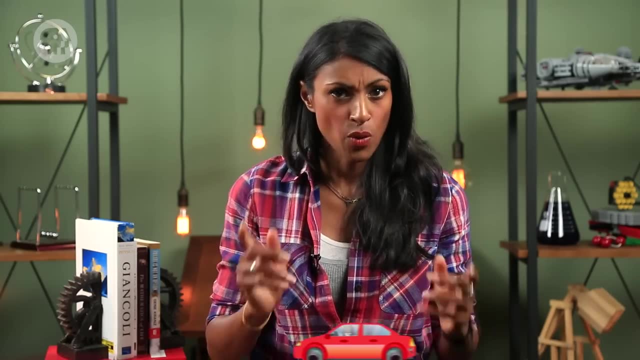 is about 214 moles. So there are roughly 214 moles of air inside your car. Now how many moles of air were inside your car when you drove home in the afternoon, when it was about 15 Kelvin warmer than in the morning? 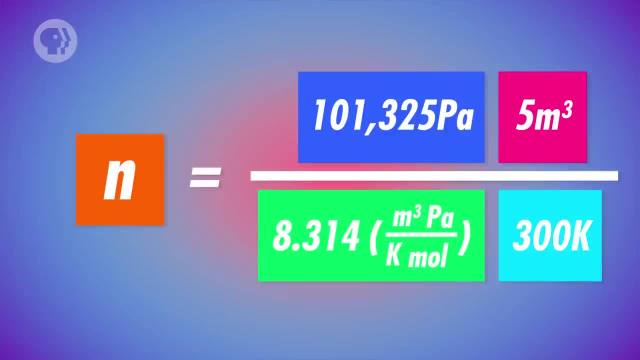 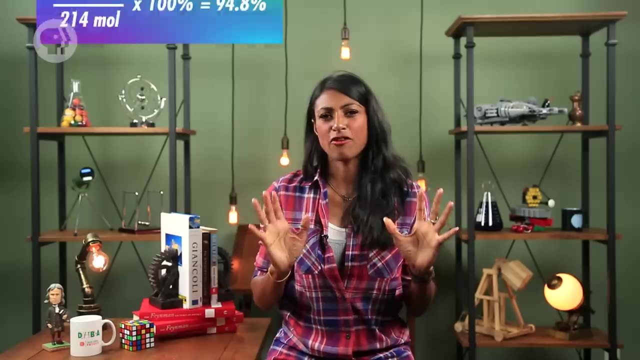 We do the same calculation, just this time with temperature equal to 300 Kelvin, and find that there are only about 203 moles of air inside your car in the afternoon. That's a difference of 11 moles. So there's about 5.2% less air in your car than there was in the morning, just because 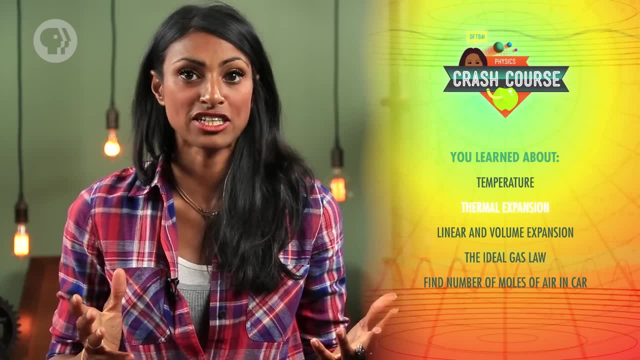 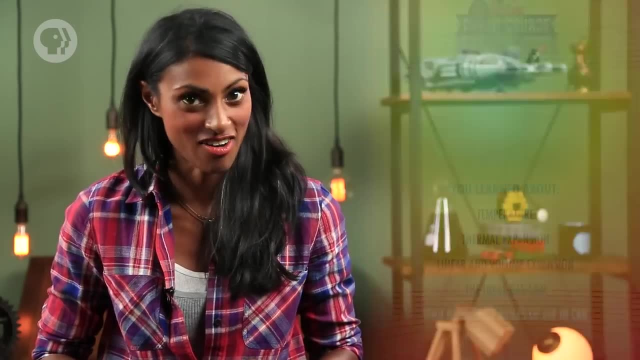 it got warmer outside Today. you learned about temperature, We talked about thermal expansion, including linear, and volatilization, And we went over the ideal gas law and how to use it to find the number of moles of air in your car. 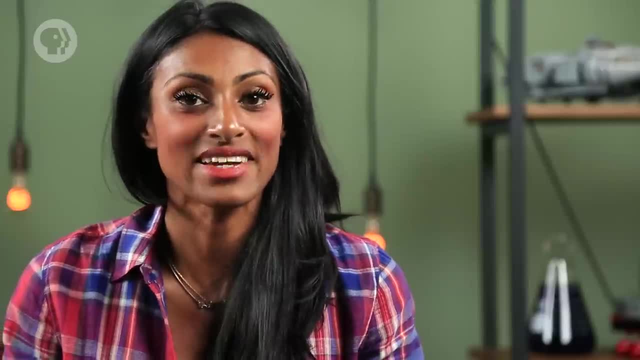 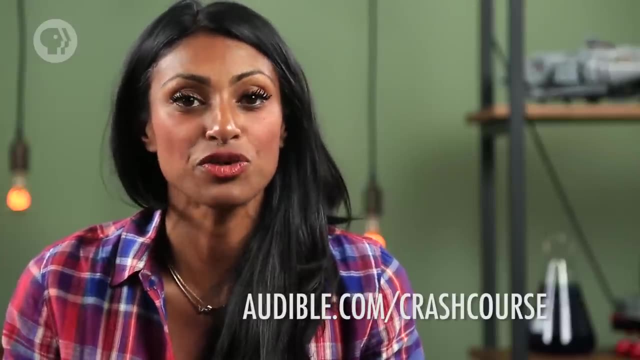 This episode of Crash Course Physics is supported by Audiblecom and right now Audible is offering viewers a 30-day trial period. Check out Audiblecom slash Crash Course to access their audio programs and titles like this book, A Brief History of Time by Stephen Hawking.